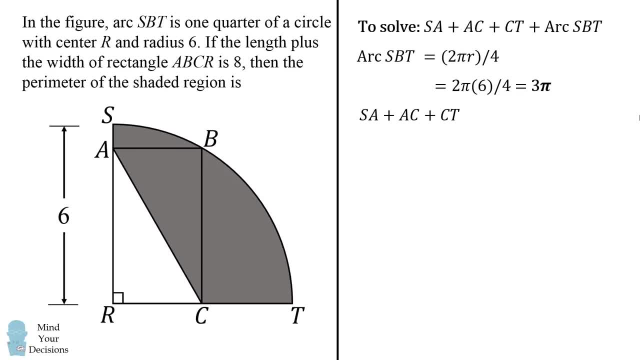 but that also seems like it would be pretty complicated. So the trick in this problem is to transform this length into the lengths of things that are already presented in the given information. The entire key is seeing that SA can be represented as the length of SR minus AR. 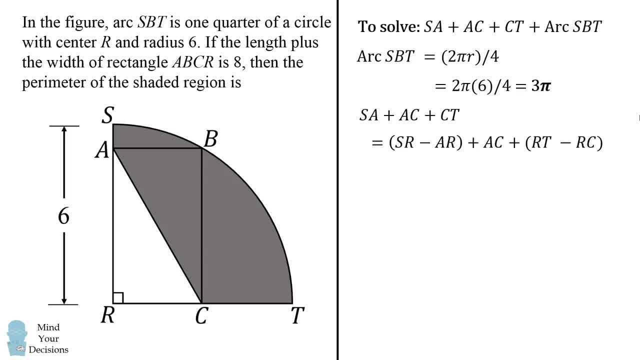 Similarly, CT can be found as the length of RT minus RC. Now, why does that help us? Well, the reason is that we know all of these lengths. So before I get to that, let me just rearrange this equation. We're going to be adding 3T. 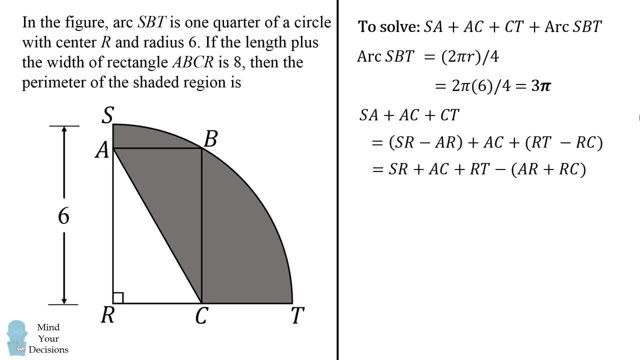 3 terms: SR, AC and RT- And we're going to subtract AR and we're going to subtract RC and we'll group them together. So we'll subtract the quantity AR plus RC From the problem. SR is equal to, RT is equal to 6,. 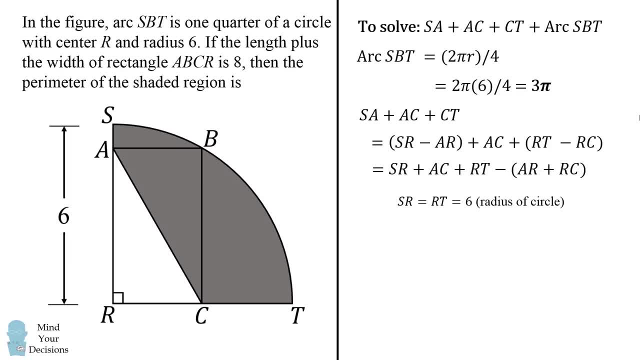 because each is a radius of the circle. Next, what about the length of AC? Well, AC is a diagonal of this rectangle, so it'll be equal to the other diagonal, which is RB, And RB is also a radius of the circle. 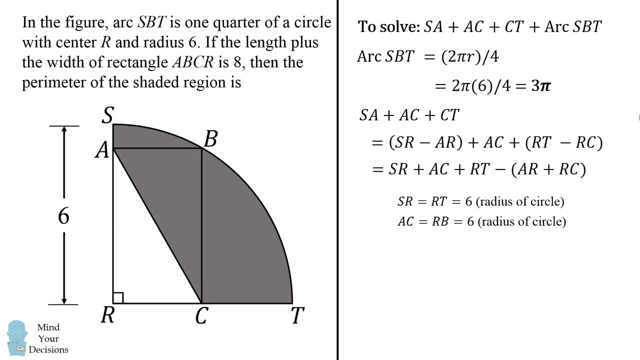 therefore, this is equal to 6, which means AC is also equal to 6.. Finally, we have AR plus RC. This is given to us in the problem as the length plus width of the rectangle, which is equal to 8.. So we now know each of these quantities. 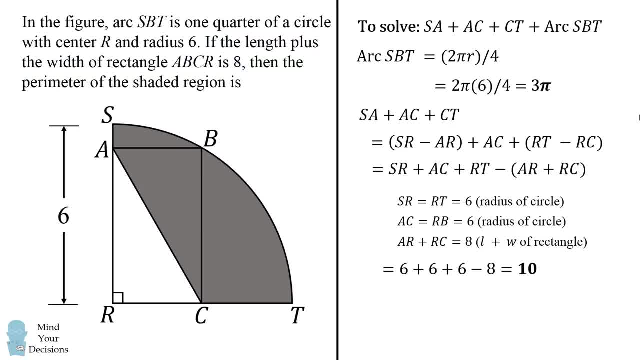 so we get 6 plus 6 plus 6 minus 8, and this simplifies to be 10.. So we put these two parts together to get that the perimeter of the shaded region is equal to 10 plus 3 pi. And that's answer choice B. 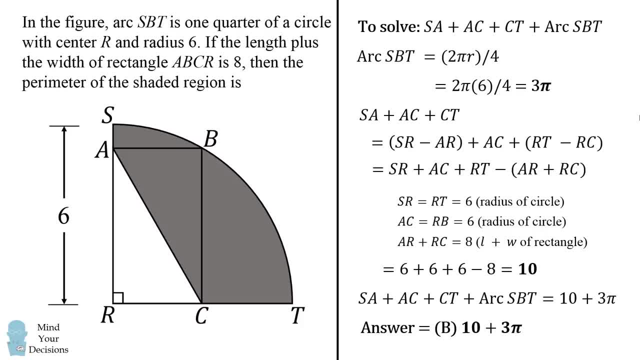 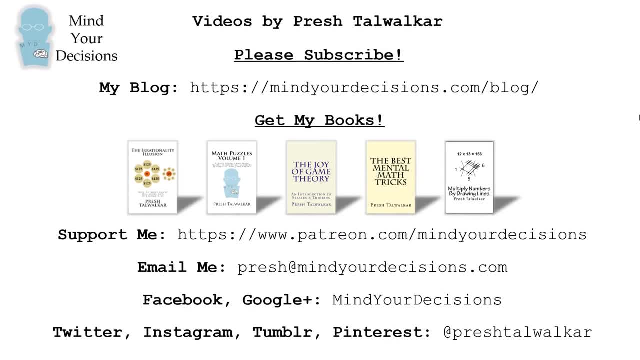 Did you figure it out And what method did you use? Thanks for watching this video. Please subscribe to my channel. I have other videos on math. You can catch me on my blog. Mind Your Decisions. If you like this video, you can check out my books.